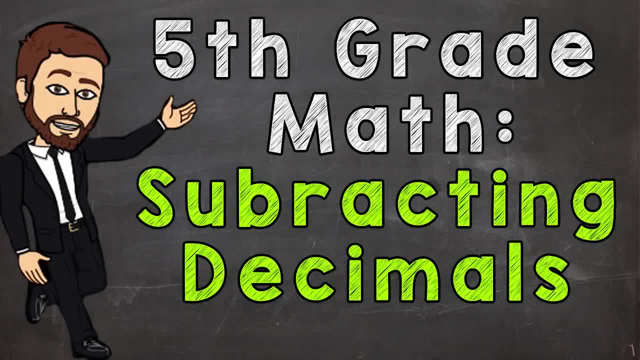 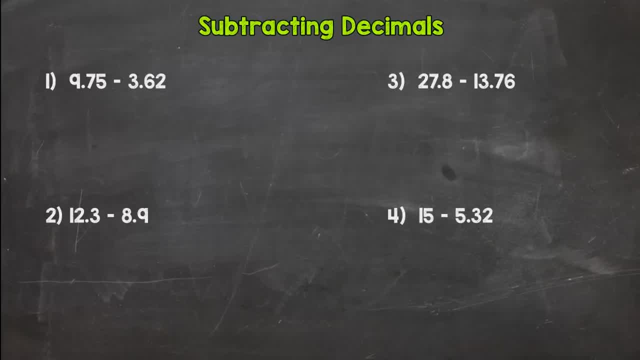 Welcome to 5th Grade Math with Mr J, And in this video we are going to be covering subtracting decimals. Now, if you have the basics to subtraction down like you know how to borrow and go through the process, subtracting decimals really isn't too bad. There's just a couple extra rules we need to keep in mind. 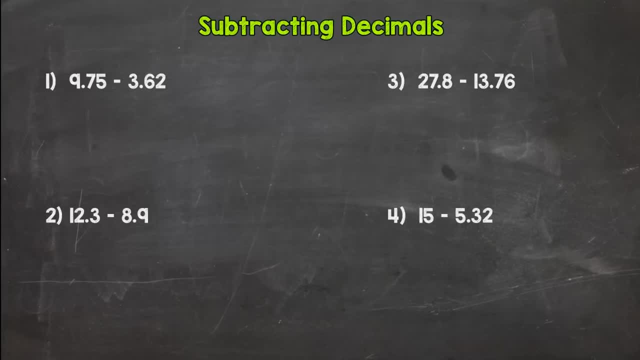 Kind of like when we did adding decimals. It was very similar to just adding whole numbers. We just had a couple extra things to remember. So this is the instructional video for subtracting decimals, where we will do the four problems on your screen together. 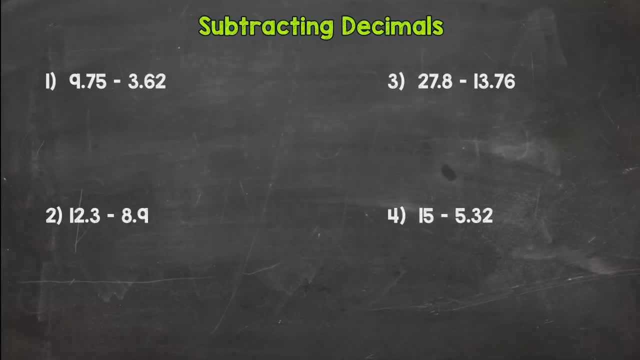 And then we'll follow this up with the mastery check, where you will do six on your own to see if you have it down. So let's hop into number one here and go through the process of subtracting decimals. I highly suggest writing these out with me, going along with me. 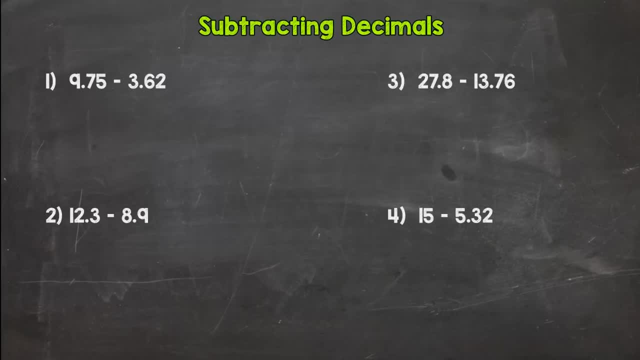 I think that will be more beneficial to you than just sitting there watching me, But either way, it's up to you. So our first thing we do when we subtract decimals is we line our decimals up Like this: Once we have our decimals lined up, we see if we need any placeholder zeros. 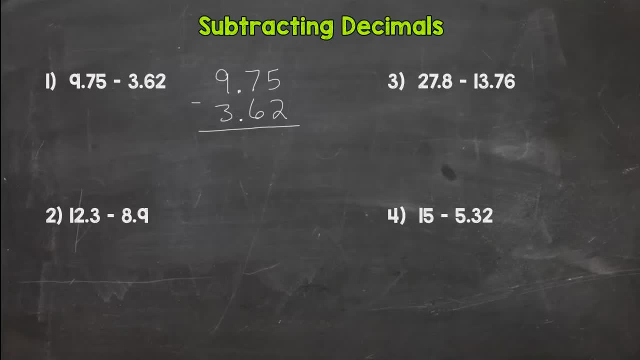 And in this problem we don't. So you'll see what I mean, if you don't, when I mention the words placeholder zeros In the following problems. But number one, we don't need any placeholder zeros. So line up our decimals, see if we need any placeholder zeros, and then all we need to do now is subtract. 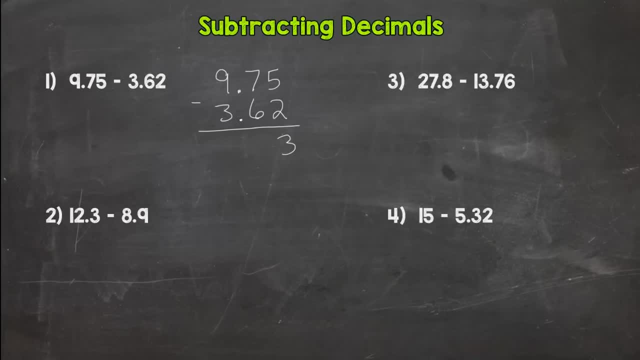 So five minus two is three, Seven minus six is one, And when we subtract decimals, just like adding decimals, we bring our decimals straight down And then nine minus three is six. So our answer is six and thirteen hundredths. Now we're going to do this again. 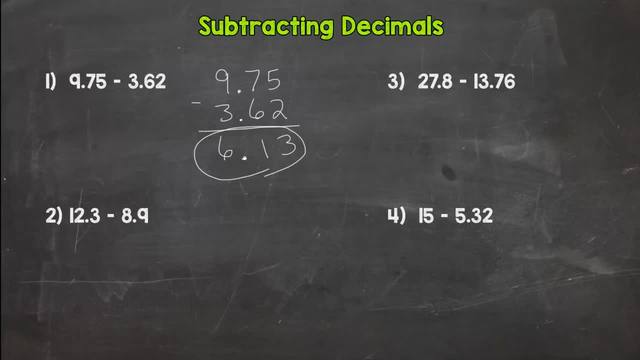 We always check to see if our answer is reasonable or it makes sense. So we're going to use estimation to do that Estimation and rounding. So I go back to my original problem. And nine and seventy-five hundredths is closest. whole number is ten. 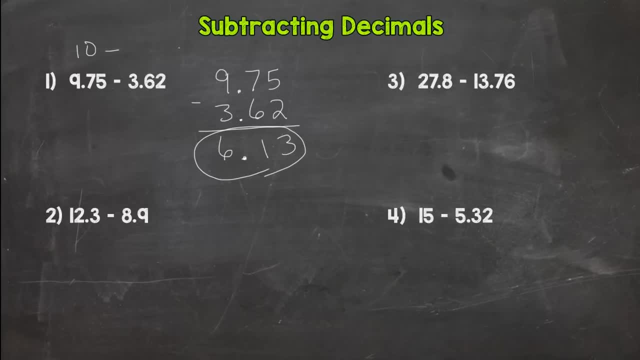 I round it to ten Minus three and sixty-two hundredths. closest whole number would be four. Ten minus four is six. That is my estimate And let's see if my answer is reasonable. Is it close to my estimate? Yes, they're very close. 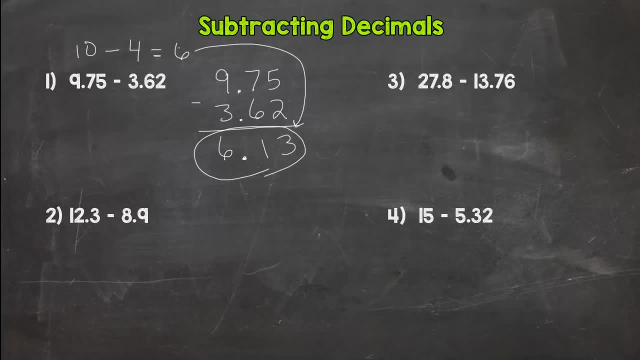 So I have a reasonable answer. Number two: What was the first thing we do when we set up our subtracting decimals problem? Hopefully you thought to yourself: line up the decimals, So let's line up our decimals, Put our subtraction sign in there. 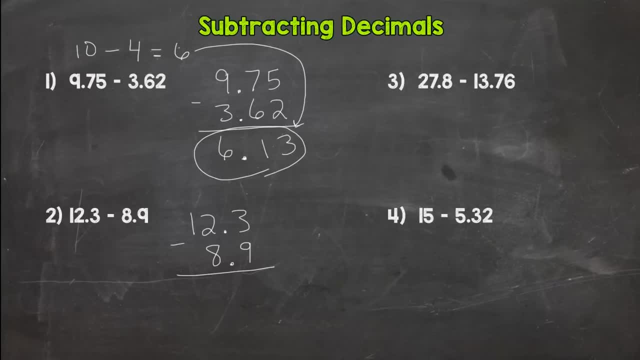 Now in number two we do not need any placeholder zeros either. But this one's a little different than number one, because we cannot do three minus nine, So we need to borrow in this one. So we take from the two and we get to thirteen minus nine, which is four. 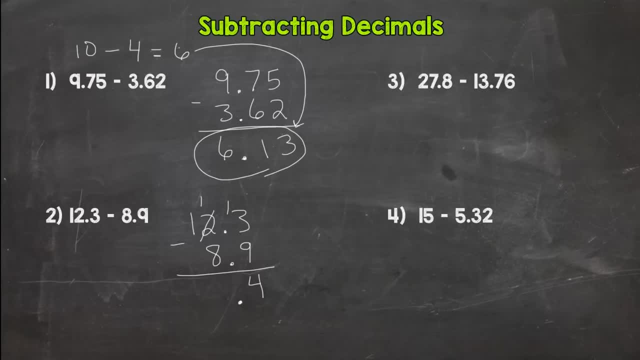 Bring our decimal straight down. Cannot do one minus eight. Don't put seven there. One minus eight is not seven. We need to borrow So we get to eleven minus eight, which is three, And then we just have a zero over there. 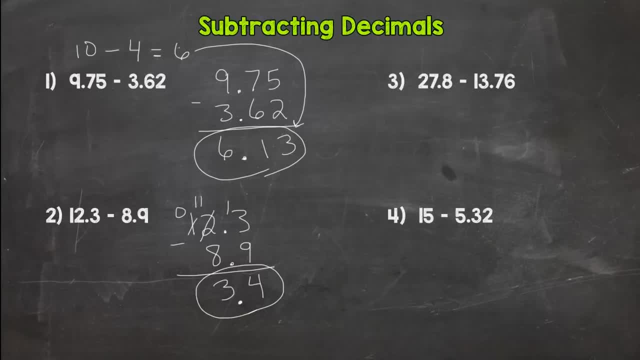 So three and four tenths And four tenths. Let's round and use estimation to see if our answer makes sense here. So this would be round to twelve, And eight and nine tenths would round to nine. Twelve minus nine is three. 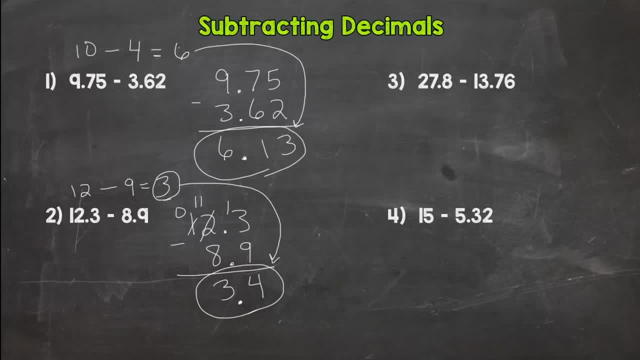 So our estimation is three. Our answer makes sense. We have a reasonable answer. Number three: First step, Line up our decimals, Put our subtraction sign, Our equal sign. Now, this one is a problem where we will use a placeholder zero. 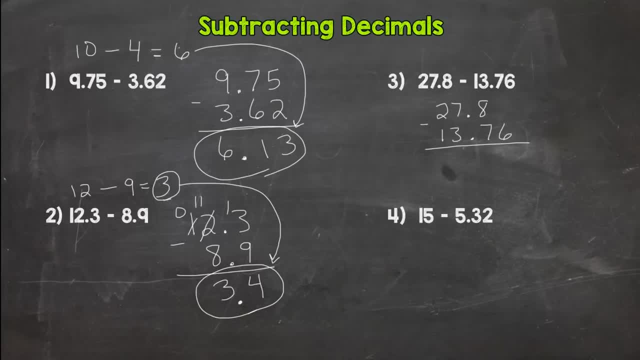 Okay, See how we're a little offset here And the bottom number has a six in the hundredths And our top number doesn't have anything in the hundredths. I'll show you the number one mistake When it comes to subtracting decimals. 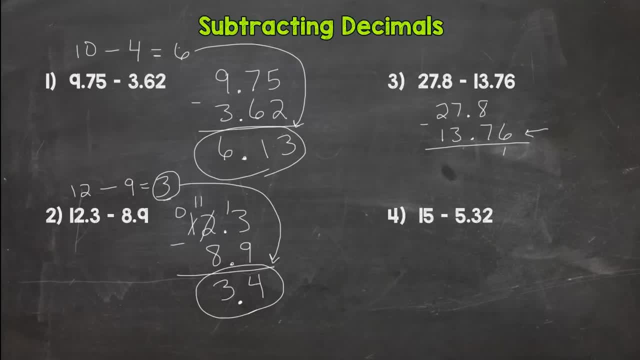 And why we need to make sure we put our placeholder zeros. You cannot just drop this six. Okay, There is a placeholder zero we put up here And we know zero minus six is not six, So this is incorrect. Don't just drop that six. 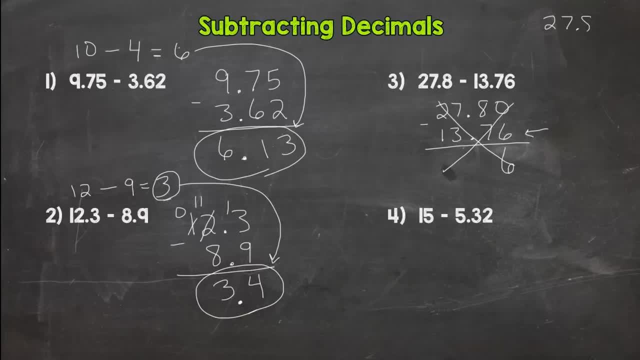 I'm going to re-line up. Up here, in the top right I put my placeholder zero. Zero minus six is not six. I need to borrow. I get a ten here. Ten minus six is four. Seven minus seven is zero. 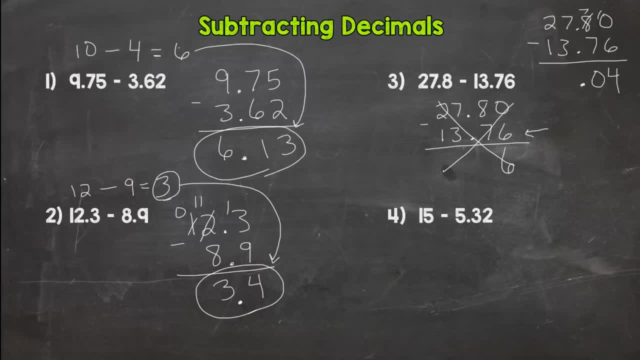 Dot, dot dot. Bring that decimal straight down. Seven minus three is four, And two minus one is one, And I get fourteen and four hundredths. Let's see if that is a reasonable answer. We have twenty-seven and eight tenths. 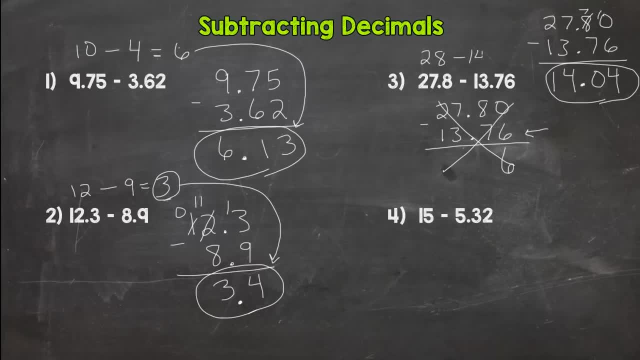 Which would round to twenty-eight Minus fourteen, Which gives us an estimate of fourteen. Is our answer close to fourteen? Yes, So we have a good answer there, A reasonable answer. Now, this helps us. Maybe you accidentally write your problem down in a sloppy manner. 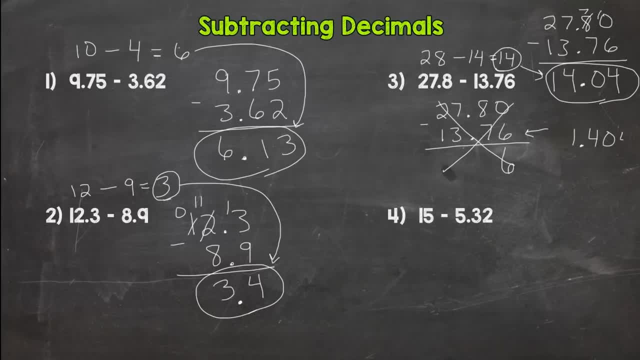 And you have the decimal right there in your answer And you go back, Do your rounding and estimation And you see that your answer should be close to fourteen, But you got one and four hundred four thousandths. That's why you use estimation. 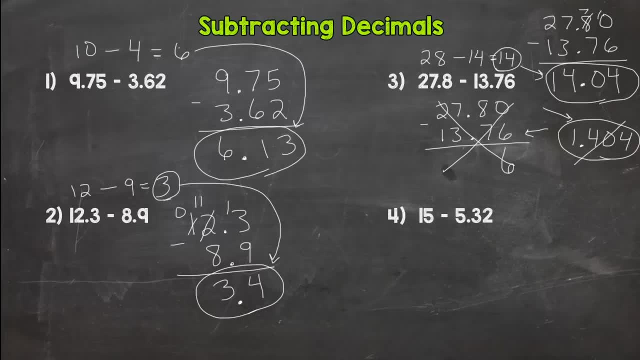 And you check to see if your answer is reasonable, Because we got something that does not make sense For something around twenty-eight minus fourteen, Okay, So check to see if your answer makes sense. And then number four here: This is a good one. 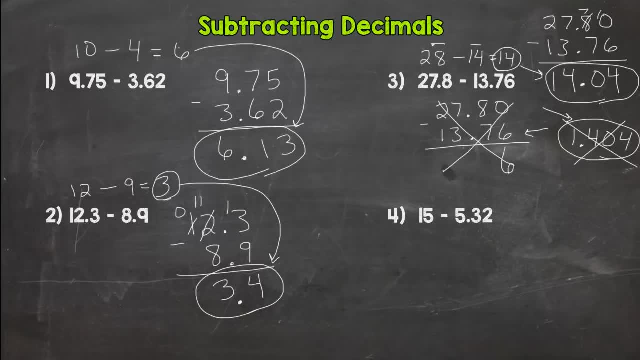 This is my favorite Because we run into one of the biggest questions I get the most here. So our first step is to line up our decimals And we have a fifteen. Well, fifteen wholes does not have a decimal. Well, actually, every number has a decimal. 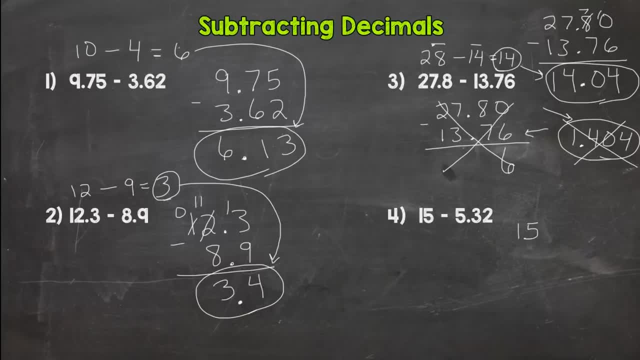 We just don't put them for whole numbers, Because it's not necessary. Think of fifteen dollars. The decimal would come right after right. Same thing for a whole number. Put the decimal right after the fifteen. Now we're nice and lined up.